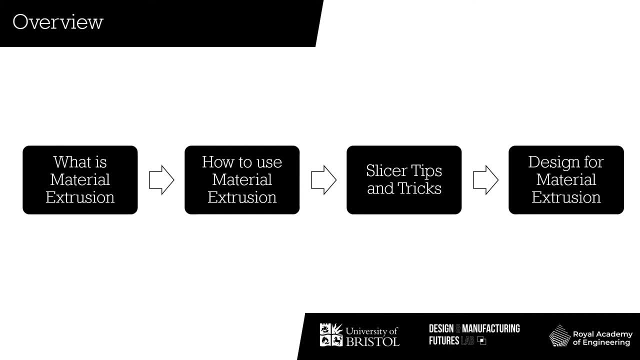 We'll then move on to briefly look at some slicer tips and tricks before finally considering some design for manufacturers approach to it for material extrusion. A set of notes will also be made available that accompany these slides for reference and further reading, as well as two posters put together by some of the DMF team. 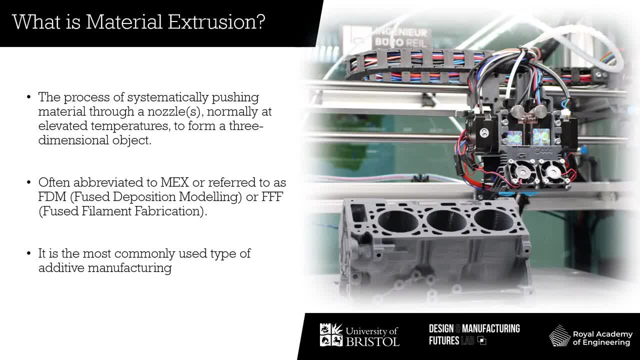 So what is material extrusion? Put simply, the material extrusion process can be described as the process of systematically pushing material through a nozzle or nozzle, Normally at elevated temperatures, to form a three-dimensional object. In the next few slides we'll have a look at how machines do this and what this means in the real. 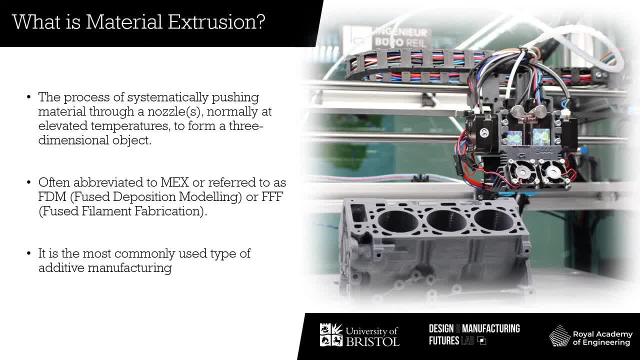 world, but fundamentally this is as complicated as the technology is. Before we continue, we should also recognise that material extrusion, often abbreviated to MEX, has many names. You may have heard the terms Fused Deposition Modelling, or FDM, or Fused Filament Fabrication, or FFF, before. 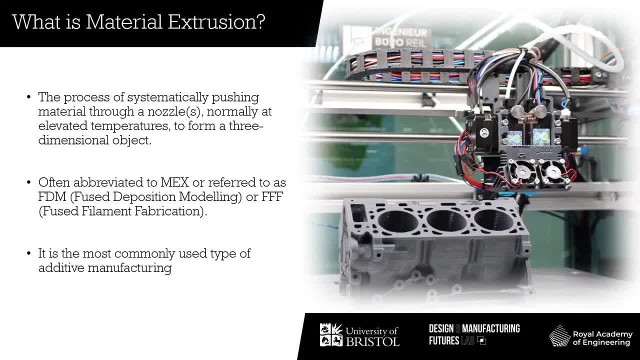 which mean largely the same thing. Material extrusion is, however, the iso-regulatory term for the technology discussed here, and so this is how I'll be referring to it throughout, though I may also use the acronym MEX. It is also good to recognise the value of MEX as the most 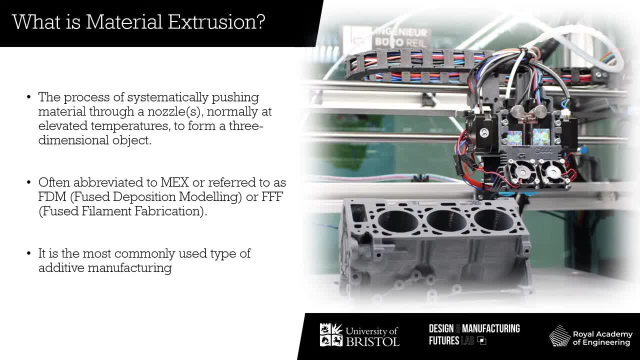 used. type of additive manufacturing, a broader term for the manufacture of three-dimensional objects through the addition of material to a substrate. Information surrounding this can be found in the annual Sculptio and WALA State of the Industry reports, along with several other sources. 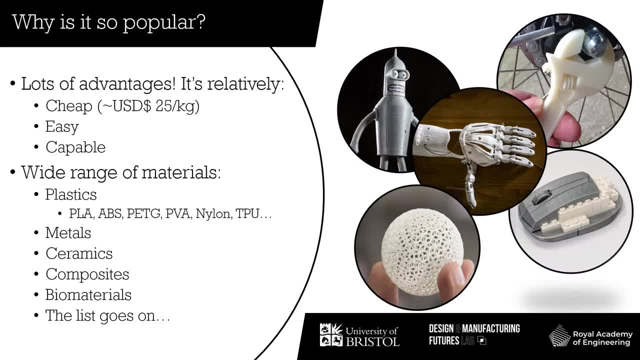 Material extrusion, as previously mentioned, is the most used additive manufacturing method around the world. It has arrived with more traditional manufacturing methods for prototypes and products for several years. Although the advantages often change or sometimes disappear, depending on what you want to print, you'll often come back to the same three: It's cheap, it's easy and it's very capable. 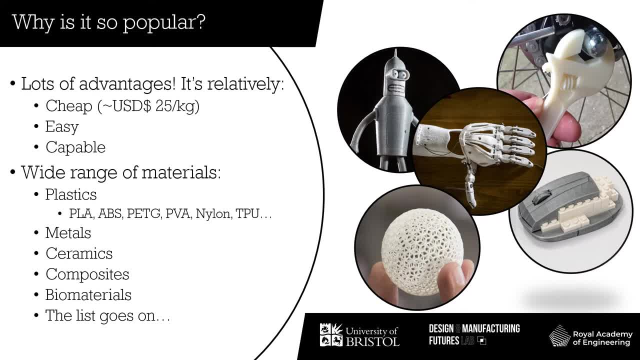 The cost of MEX has been reducing consistently now for many years as progress is made, developing consumer-grade machines, which now start from just $200.. Along with this, the most commonly used material, PLA, can be purchased in a suitable format from around $25 a kilogram. This helps. 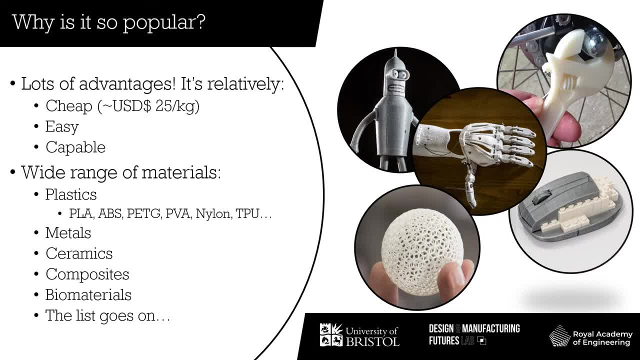 to reduce the barrier to entry, which is already quite low because, compared to lots of advanced manufacturing processes, it's so easy. We'll go through the process in more detail later, but for lots of users the print process can be as simple as turning the machine on, opening your model and 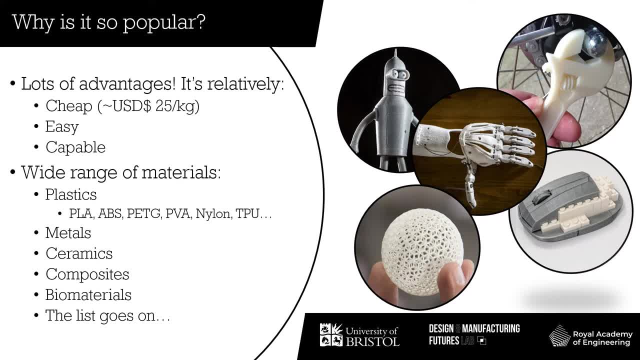 pressing print. The technology is very capable too, As you can see from the pictures on the right and for hundreds of pages on Google, Reddit and the rest of the internet. the geometry an MEX printer can produce are incredible and can realistically only be matched by other additive. 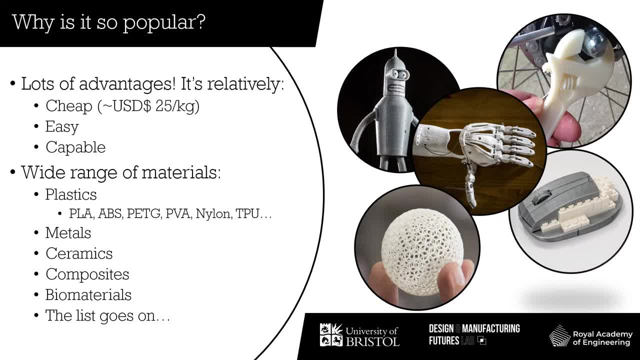 manufacturing methods, Though I will take a second here to note that there are still limits, which we'll come onto later. Finally, the choice of materials available has made several people and companies take note and adopt the technology. Firming plastics remain the most widely used materials when using MEX. 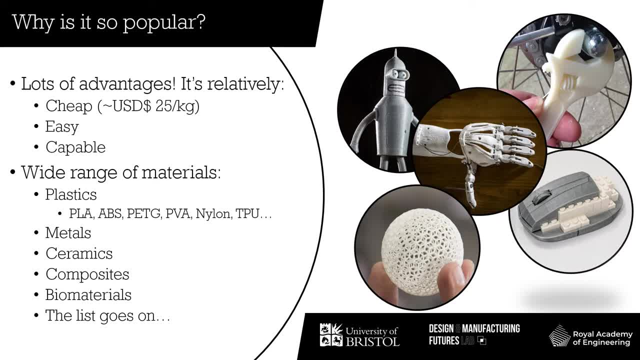 generally due to their ease of use, relatively low melting temperatures and cost. However, we've started to see applications of a lot of different materials. You may recently have seen companies printing houses in the news. That's pretty much the same process. Not only this: you can print in metals, other ceramics. 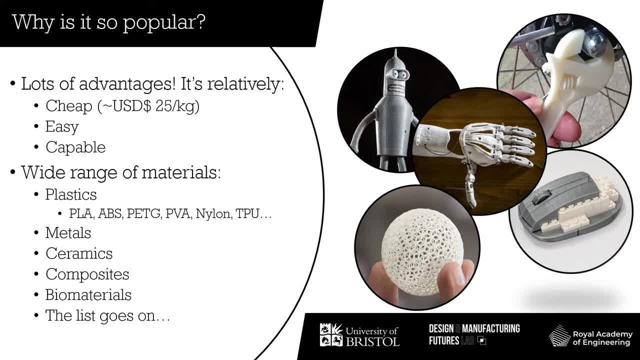 composites such as fibreglass and carbon fibre, and biomaterials and foods. Have a Google. it's incredible what people have tried. For most work, however, firming plastics suffice, especially when you just want to see what a design looks like in the flesh. As such, 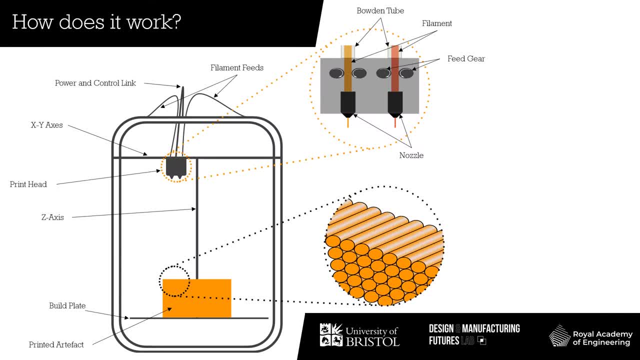 this is what we'll focus on for the rest of this video. So now we come on to how does the technology work? Although this diagram may look complicated, the technology behind an MEX printer is actually quite simple. You normally end up with a printhead attached to a set of axes that allows motion in. 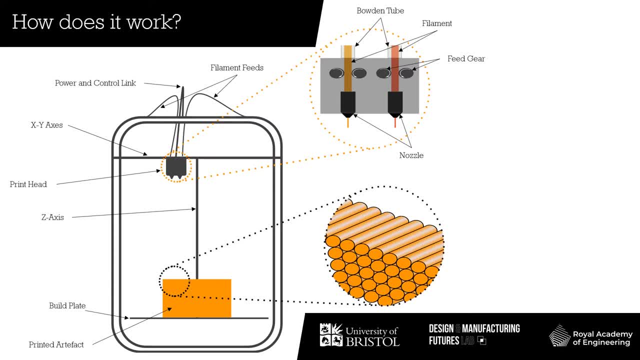 three dimensions. You can also use a printer to print a set of axes that allow motion in three dimensions. You can also use a printer to print a set of axes that allow motion in three dimensions. You then attach the printhead to a set of motors, normally stepper motors. 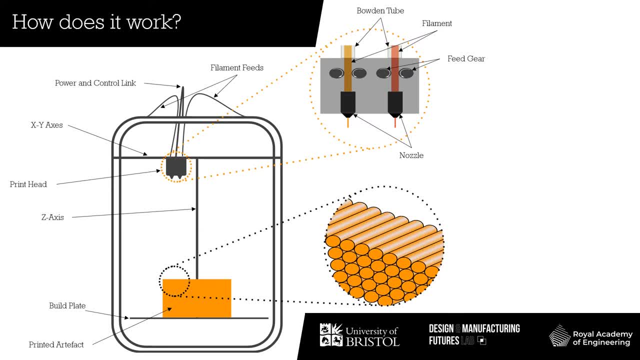 and a control system that allow the printhead to move in each axis. This allows for three-dimensional material deposition. Of course, you need to have material to deposit for this to be any use, and this is done through the use of filament- long wire-like reels of material of a constant diameter. Filament is 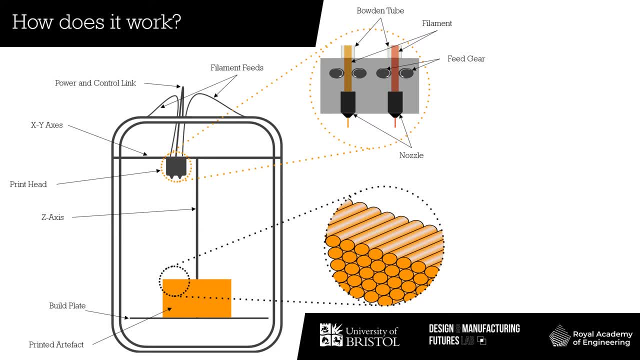 fed into the machine using a set of gears and motors that are linked to the same control system as printhead translation. By doing this, the rate of material deposition can be carefully controlled as required. As the filament is fed into the machine, the material is heated in the printhead. 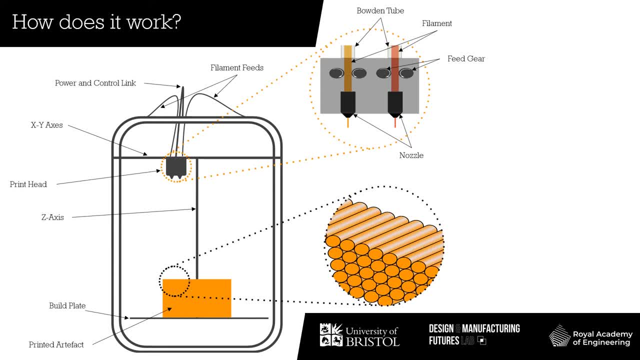 and melted to form a melt pool before passing through the extruder and through the nozzle. If the nozzle position is correct, the material should then be deposited and lightly pressed into a substrate or previous deposition, As the deposited material cools a solid 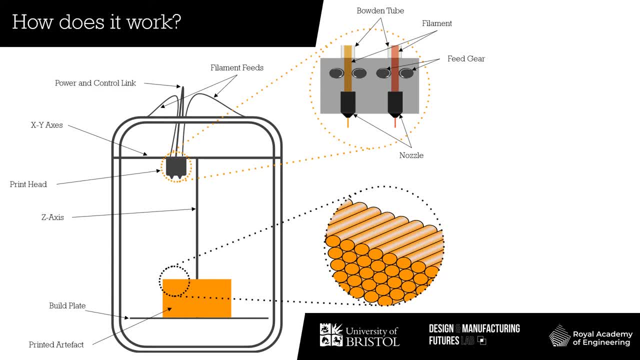 is formed in a similar geometry to that deposited. It's important to note that not all MEX printers will look exactly like this, nor have the same configuration. For example, the Automaker series of printers place the feeder mechanism away from the printhead to reduce. 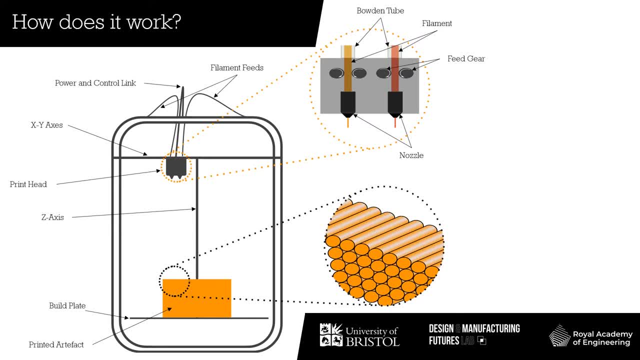 printhead mass and allow for finer control over the XY position. In comparison, the MakerBot printers often have the build plate move in the X direction, so the printhead only moves in Y, again for accuracy reasons. Here we have a brief, very brief selection of MEX machines. 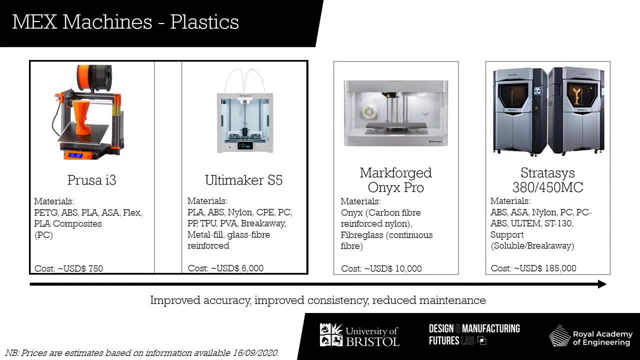 all of which are designed for printing plastics or variations thereof. I previously said the machines start at $200, and they do, but, as you can see, there's a wide range of prices, with the Stratasys 450MC, as an example, at $185,000.. Of course, what the $200 machine? 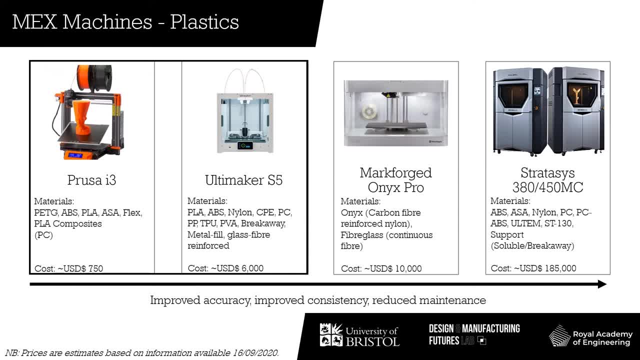 and what the $185,000 machine are capable of are quite different. Much of the improvement that is achieved in the more expensive machines comes from more rigid frames, improved control of the printhead or build plate or better temperature control, though there are often several other advantages too- The Markforger Onyx Pro, for example. 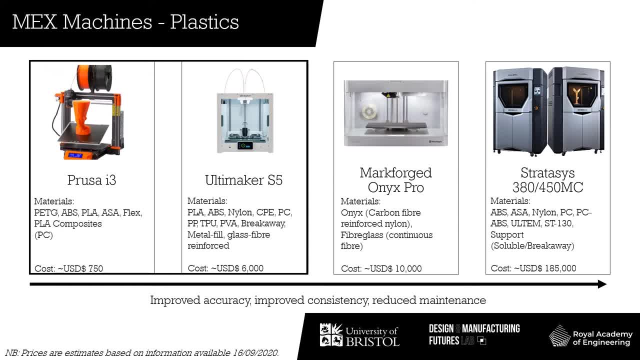 allows the user to use proprietary materials that allow continuous glass fibres to be placed in the part for improved strength. It's hard to explicitly say what machine is best for any given task, but most commercial users and students will find that machines at the lower end of the 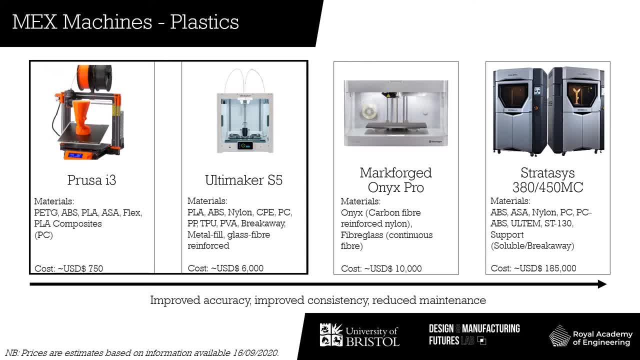 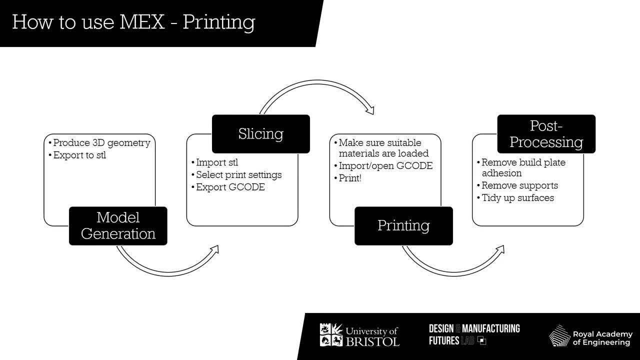 scale will suffice for prototyping applications in thermoplastics. The printing process can be easily devolved into four key steps: Model generation, slicing, printing and post-processing. We'll go into a little bit more detail for each of these steps in the coming slides, but the process can be quite simple with much of the work automated. 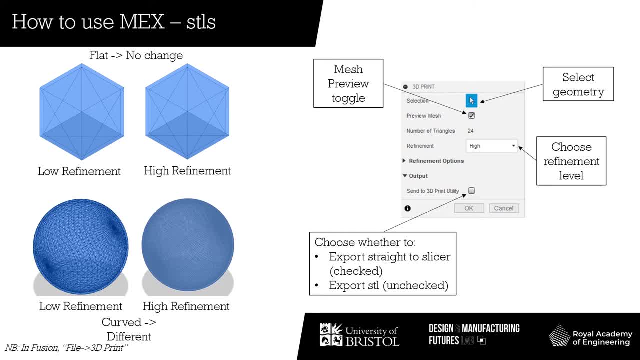 STL files are the go-to file format when 3D printing, allowing the user to easily produce a surface representation of a solid body that can be used in the printing process. Most CAD programs, and all I've encountered, allow the user to export a body or bodies. 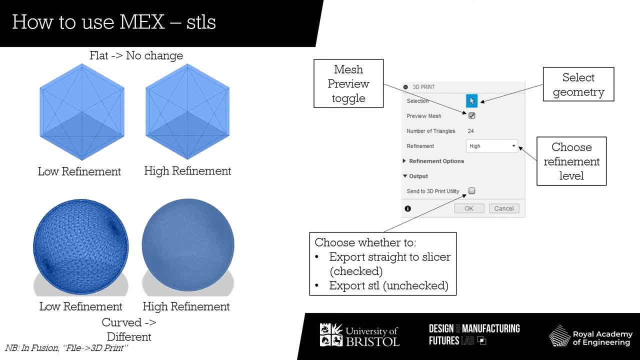 as an STL, though some allow for greater control over settings than others. For some models, the parameters used in the STL generation will not significantly affect the model printed, which is a good thing. However, if the model is printed in a 3D printing environment, the 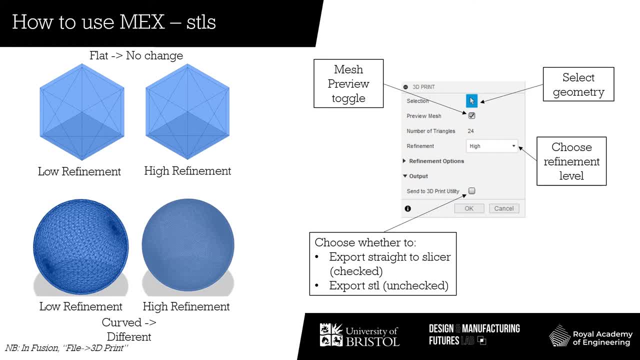 error in the print will be a lot greater. However, as printers improve and for models with lots of complex curved surfaces, the errors associated with generating the STL become more important considerations. Fortunately, Autodesk Fusion has provided the user with several STL settings that can be adjusted to suit a user's needs. The basic settings menu from Fusion can: 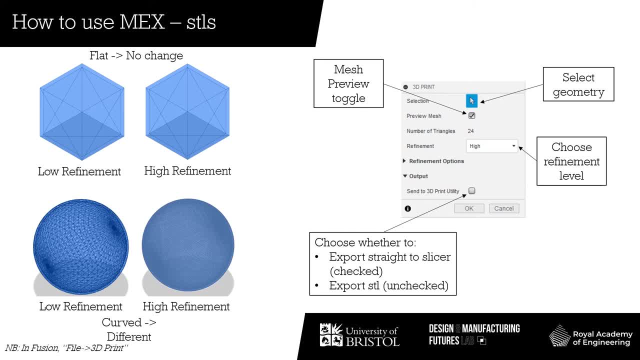 be seen on the right of your screen. This menu can be accessed by going to File 3D Print. Note that going to File Export and selecting STL is not the same process and will result in you having a little less control over the model. However, if the model is printed in a 3D printing environment, 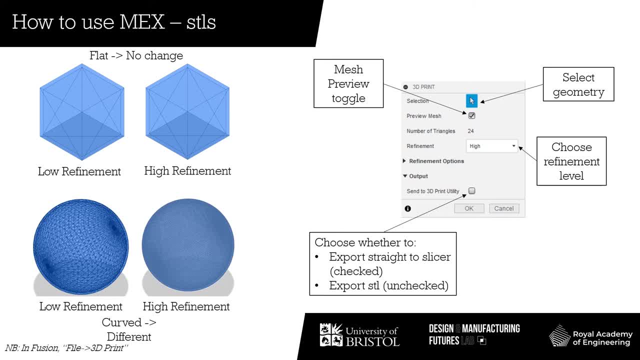 you will have less control. It also takes longer on most computers, so I would strongly encourage the use of the 3D Print Utility. In this menu the user can select the bodies to be converted, choose to preview the mesh, choose a refinement level and select whether a 3D Print Utility 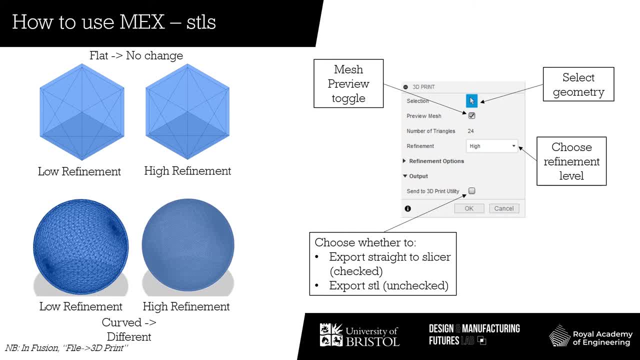 should be directly exported to. Most of this is quite straightforward and there are lots of videos available online that show how this can be used, but I wanted to highlight the importance of selecting a suitable refinement level for your model. On the left of your screen, you can see a cube and a sphere as an STL representation. 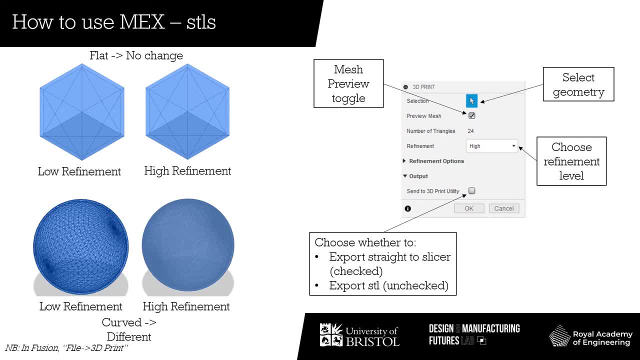 using low and high refinement. Hopefully, you can recognise that the cube can be defined very easily using tessellated surfaces, with two triangles required for each surface. As such, there is no significant difference in the STL representation whether using low or high refinement. 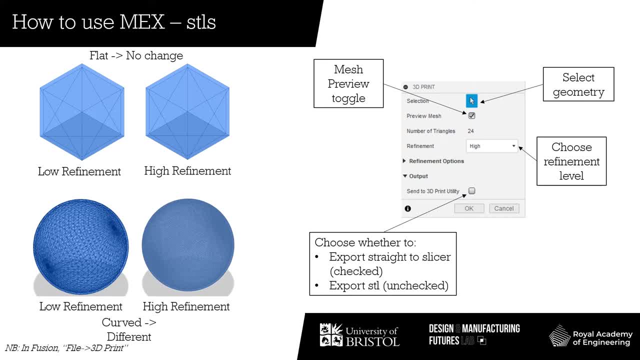 However, the sphere shown has a very different mesh for the two refinement options. This is because there are no flat surfaces in a spherical body and therefore a triangular surface representation introduces error As such if the program is allowed to generate triangles with a. 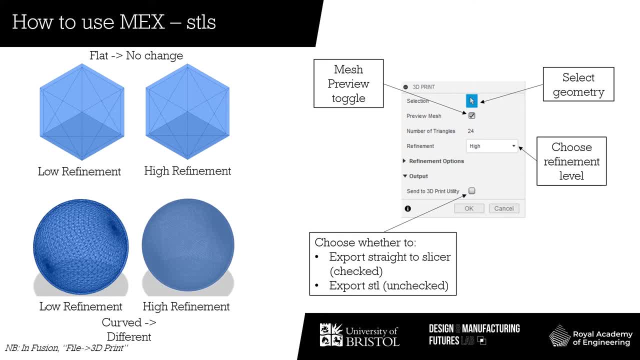 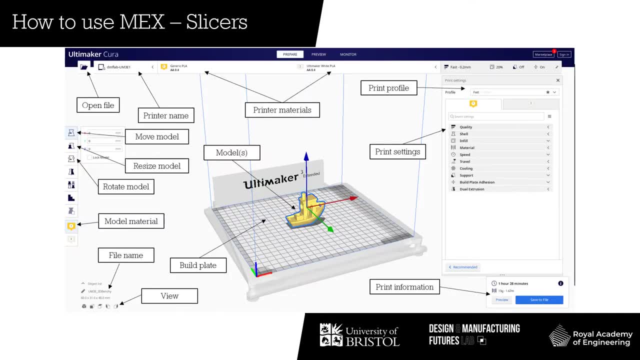 smaller edge length, a more accurate representation is produced. It is for models such as this, with high levels of curvature, that choosing a suitable level of refinement is most important. Once an STL is produced, the next step is to use a suitable slicing software to slice your model. 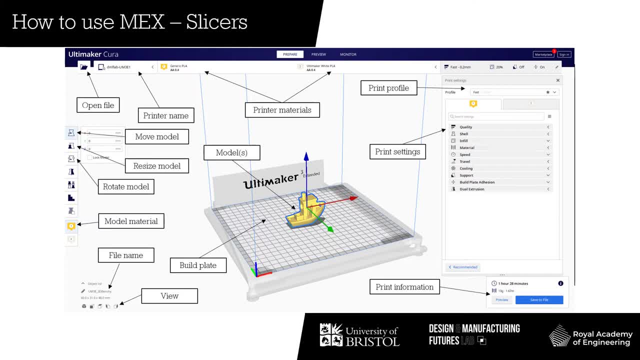 and produce a file a 3D printer can understand. Shown on the screen is a screen grab from automaker Cura, with the Benchy test print on the build plate. Cura is an open source slicing software that is freely available online, though it natively is intended to support the automaker. series of printers. Cura is an open source slicing software that is freely available online, though it natively is intended to support the automaker series of printers. Cura is an open source slicing software that is freely available online, though it natively is intended to support the automaker series of printers. 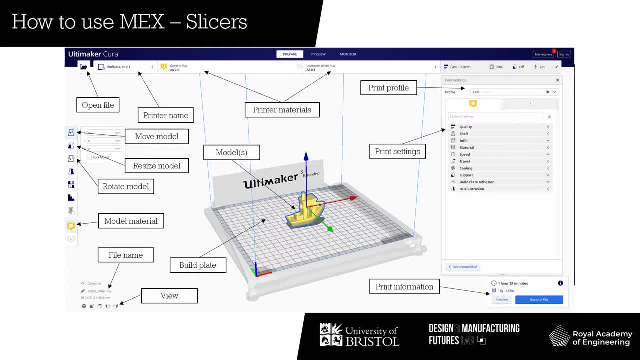 There are lots of profiles available for other printers and the user is also able to set up their own in the software. This can be done by clicking the printer name box shown. Other slicers are also available for free and for a fee, so it's generally up to the user what they 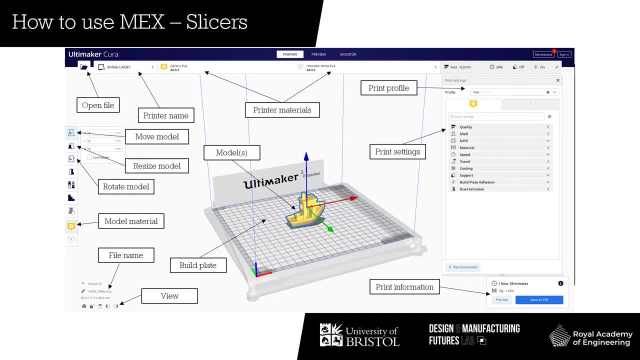 use. Some printers also have proprietary software which you may be forced into using. I'm not going to go through every mode and setting that can be changed in Cura. You're better off searching for what you need in the internet or in your slicer's manuals. However, I will point out a few key points. 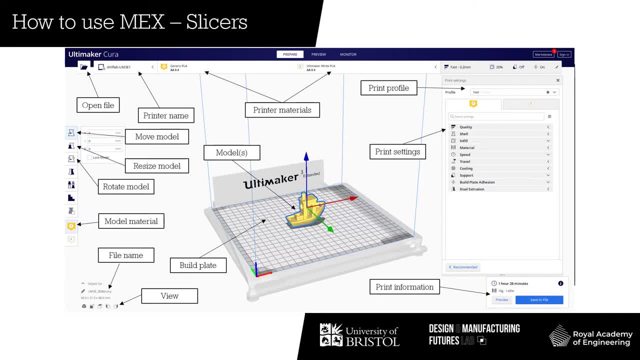 Firstly, you will want to bring in your own STL file or files. To do this, click the folder in the top left hand corner and search for the file, or just drag and drop the file into Cura. Once this is done, you will see a menu on the left hand side of which the top three options are important. 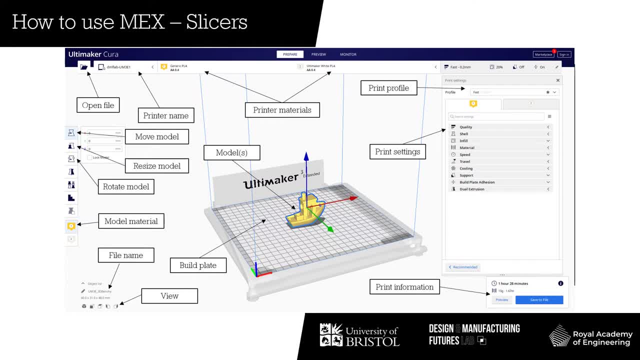 Move Model, Resize Model and Rotate Model. Further down, you'll also see Model Material which, if using a multi-material printer, will let you choose what material the model is printed in. The materials shown here are dictated by what's the file size. 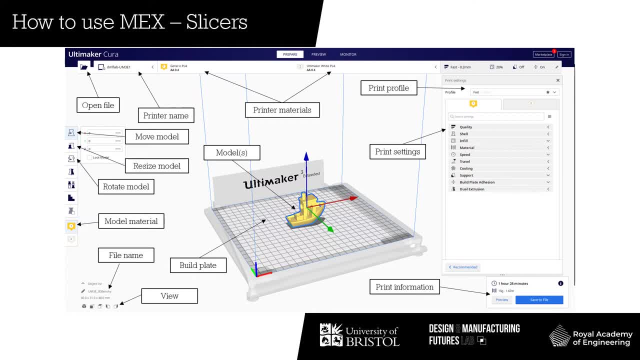 In the bottom left corner you'll see the file name, which you can change, and a choice of views. On the right hand side of the screen are the printer-specific profiles and print settings that can be changed. Generally, you'll want to stick to the default Cura profiles. 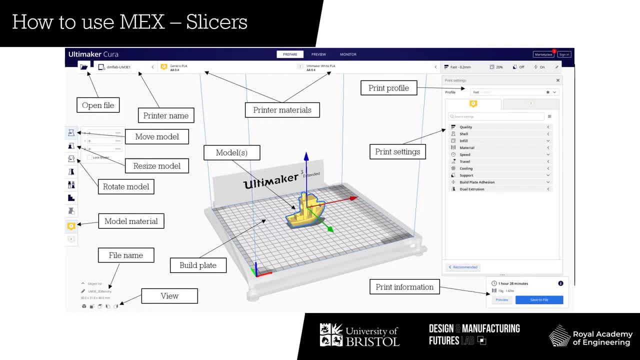 or profiles given to you. That will be fine for pretty much everything you print. However, if you want greater control over the output, you're able to change almost any setting you might want to from the drop-down lists available. Finally, in the bottom right hand corner, you'll 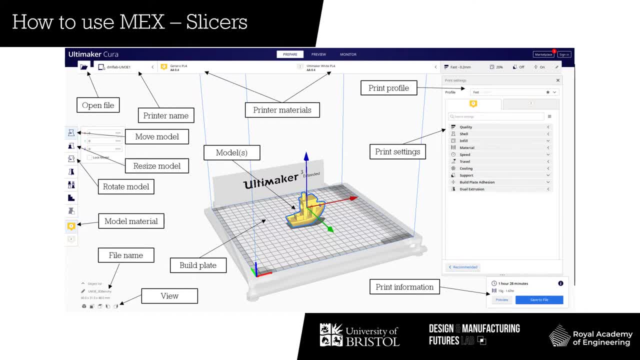 have your print information, though you may need to slice the model before seeing this. In this box there will be a print time estimate, along with estimates for material mass and filament length After slicing your model, I would strongly suggest that you check the preview screen in Cura. 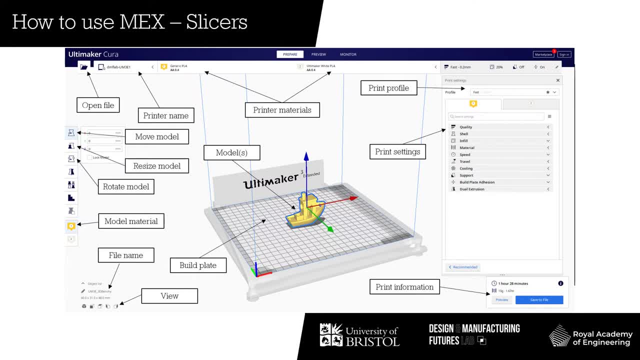 found just above the print materials. In the preview screen you will see a layer-by-layer, extrusion-by-extrusion breakdown of the print. that will give you a good idea whether your print will work or not. If you're not happy with anything, you can go back and fix this at that point, Rather than 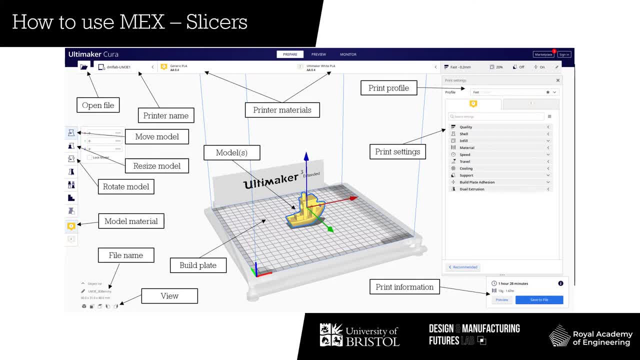 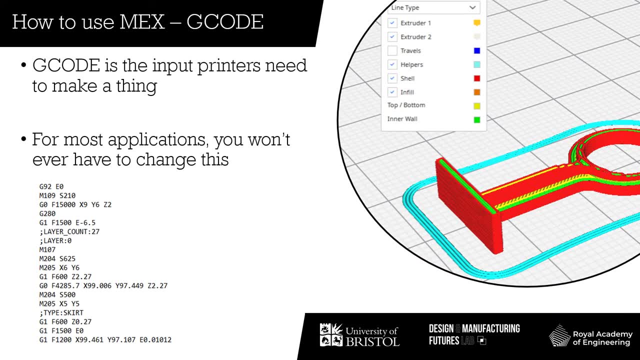 waiting for a print to be ready for hours or days. If everything's good, though, you can export the file or send it directly to a printer. Once you've exported the file from Cura, you will have a G-code file or a version of G-code, depending on your printer. 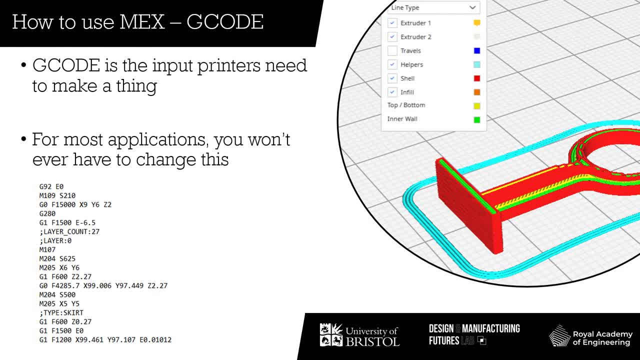 G-code files are basically lines of text with G or M codes that a printer can interpret and act upon. There is lots of information available as to what different codes mean online, so I won't discuss this, But I wanted to highlight that you can bring a G-code. 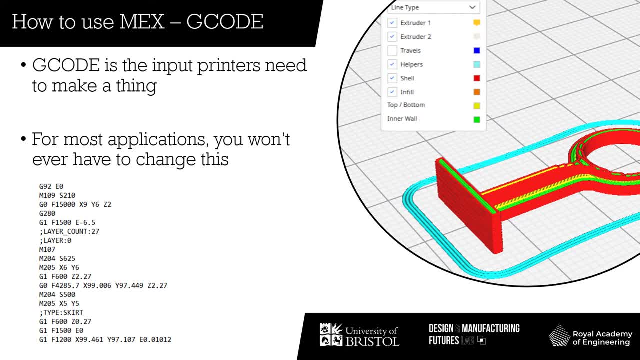 file back into Cura and get an equivalent view to the preview tab previously mentioned. This is a particularly useful feature if you can't remember what a G-code file looked like or you want to check some code before loading onto a printer, Because G-code is just text. a user is able to change G-code by hand or automate the process. 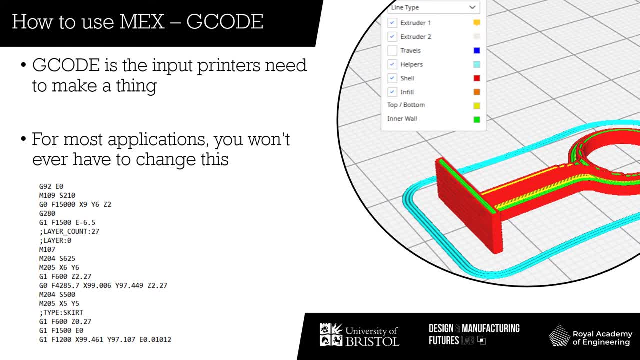 fairly easily. However, it is unlikely that you will have to worry about this, with Cura providing great enough flexibility that most parameters can be changed more easily in the slicing software. What also understanding G-code also does is highlight that printers are generally stupid. 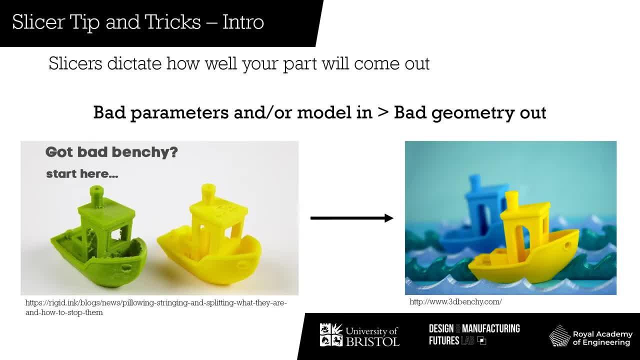 In the next section of the video, we're going to cover a few tips and tricks regarding slicers. However, it's important to note at this stage, as we've just seen, MEX printers are stupid. They'll print whatever you tell them and, with very few exceptions, won't stop. 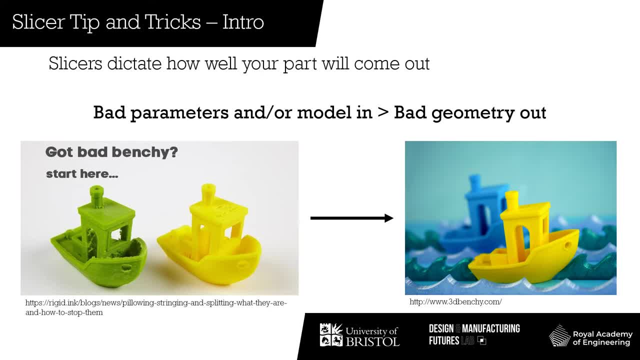 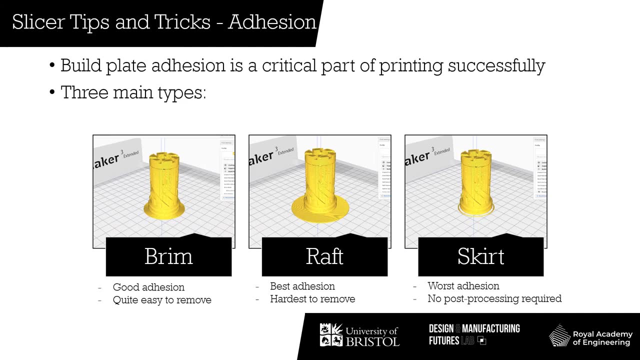 if, when something goes wrong. Not only this, but the part performance, material usage and print time are all directly derived from what you, the user, input. As such, it's incredibly important that you provide the right inputs. The first of our tips and tricks focuses on build plate adhesion. 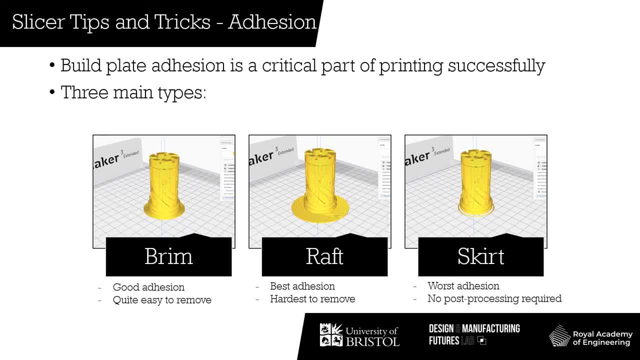 which is of paramount importance when printing parts on MEX printers and is probably the main failure mechanism you'll come across. Most slicers have three main adhesion methods: brim, raft and skirt. though they may have different names, As you can imagine, each of the methods are a lot like they sound. 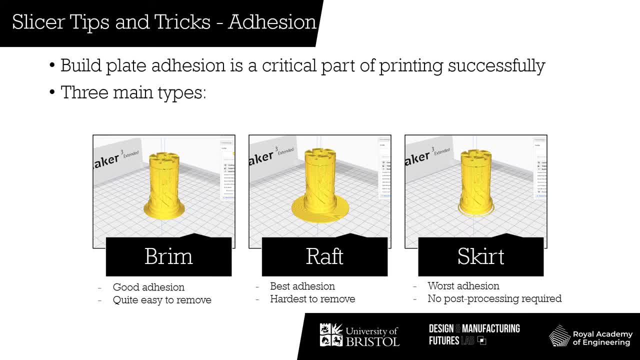 Brim prints a brim around the part to increase the surface area on the build plate. Raft prints a raft under the part connecting the part to the build plate. This can be particularly useful when printing on an unheated print bed. 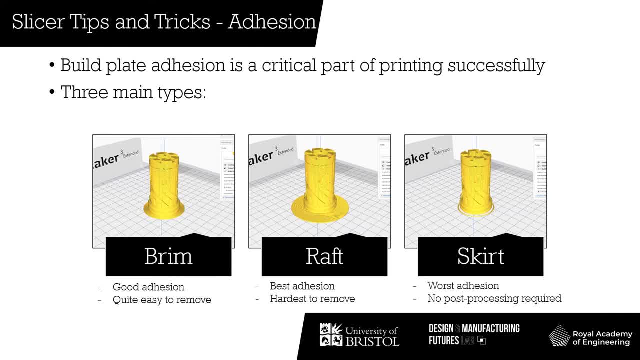 And the skirt method prints a small skirt around the part without there being any contact with the part itself. This doesn't directly improve the print bed adhesion, but is a useful way to prime the model and make sure the print bed calibration is suitable. 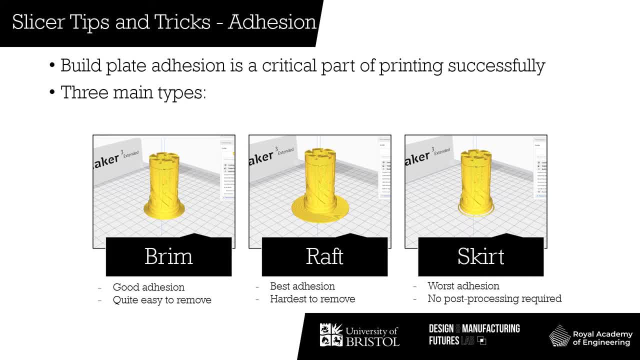 Each of these have their own pros and cons. Generally, there's a balance between cost, time of manufacture, print, bed adhesion and time required for post-processing. It's up to the user what they would want to use with part geometry and purpose. 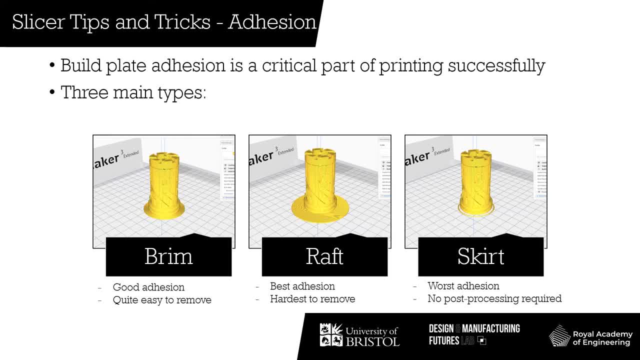 likely to be the driving factor. The default cure profile is used a brim adhesion method and this is what I would suggest. most of your prints are left as. However, if you're printing parts for late stage prototypes, you may want to consider trying to print with skirt to improve the look of your parts. 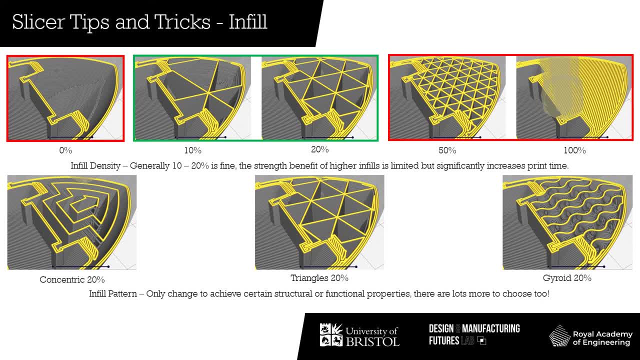 The infill density and pattern are other parameters you may want to change. Those of the faults used in most slices are generally suitable for most parts. You'll likely find that slices will generally suggest somewhere between 10 and 20% infill and this provides a good compromise between print time, part strength and supporting epicentre. 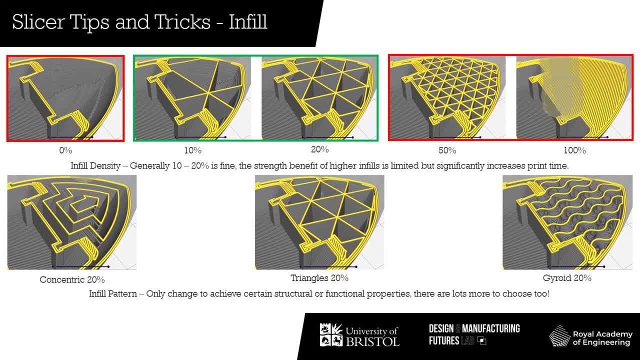 upper surfaces. If 0% infill is used, you may encounter issues with part strength and unsupported surfaces- discussed more later- and so the saving of print time and material will be offset by increased print failures. In contrast, infill densities above 20% will slow the print time down. 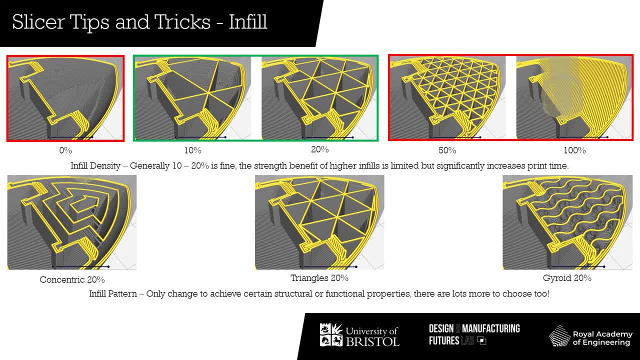 increase cost and make your part heavier without increasing your part strength significantly. The only time I'd suggest you change the infill density is when printing for a specific application, such as when printing with flexible materials to achieve specific part strengths for which you have done some modelling, or when completing research specifically into the effects of infill. 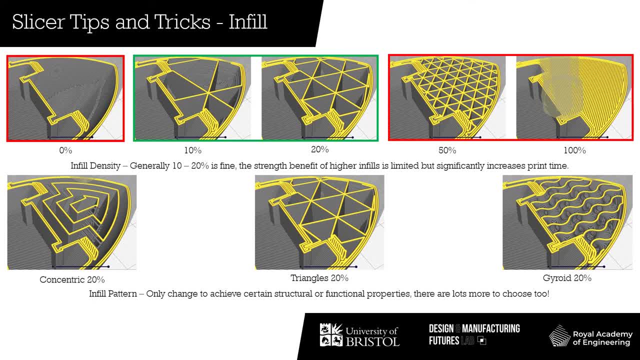 density. In a similar vein, you are able to change infill pattern to one of many different patterns that are available to the user. Generally, this should only be done for very specific reasons, such as to manipulate structural properties or utilise the infill structure to add functionality. 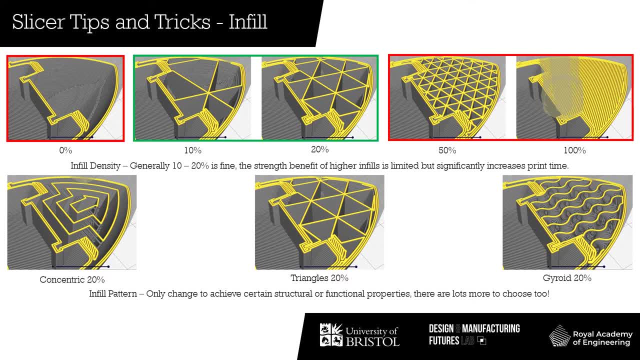 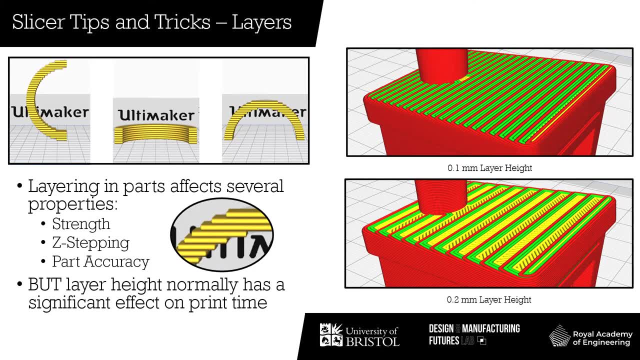 One potentially useful infill pattern to be aware of is gyroid, which aims to provide an isotropic internal structure to parts sliced and cured. Material extrusion is a layered manufacturing method that can be used to create a material extrusion As such. you will normally see some level of Z-stepping when printing parts. 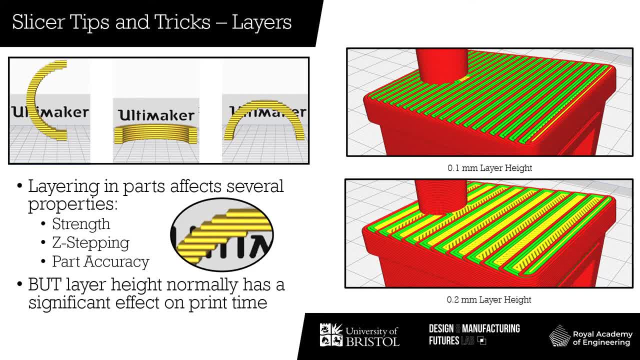 where parts are changing cross-sections relative to the Z-axis demonstrates staring on the external geometry. You can see this in the top left set of images. If you orientate your model such that the cross-section is consistent, you won't see this effect though, so keep that in mind. 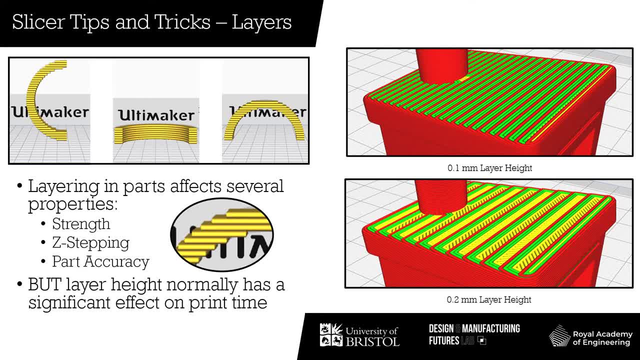 Whether you think you will see Z-stepping or not. one of the key parameters you need to consider is the size of the layers that are deposited. For most desktop MEX printers, layer heights are generally in the region of 0.1 to 0.2 mm. For most desktop MEX printers, layer heights are generally in the region of 0.1 to 0.2 mm. 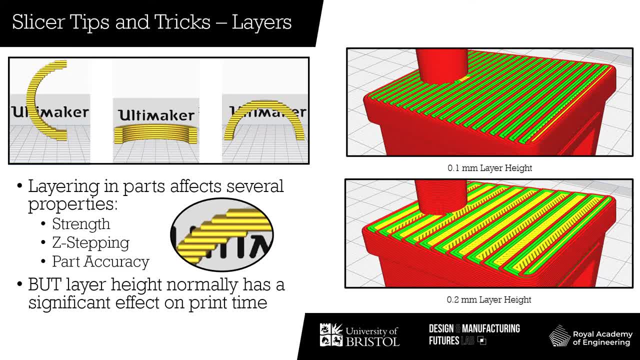 for most desktop MEX printers, layer heights are generally in the region of 0.1 to 0.2 mm. It is highly advisable to stay within the recommended limits for the printer you use, as you will likely see the best results possible. 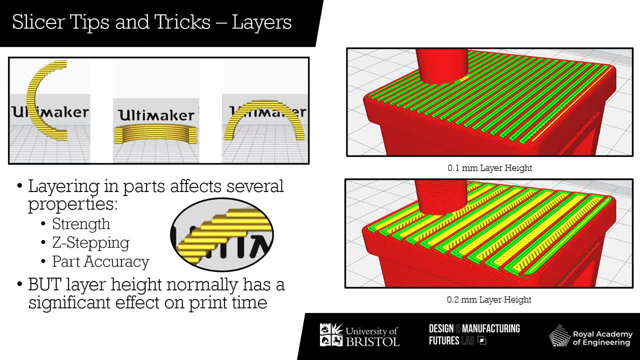 To choose a layer height within recommended bounds. however, there are many things you need to consider. The obvious two are part accuracy and 3d and printtime, which need to be balanced depending on the resources available and the required accuracy. There isn't a general rule of thumb for this, as every situation is different. 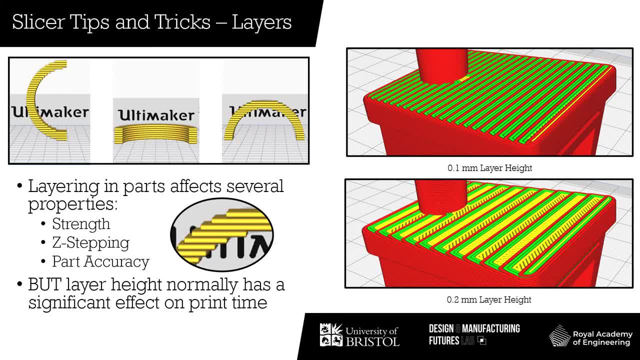 so you should consider what is suitable for you. You should, however, consider the minimum feature size you have in the z-axis. If you have a tight z-axis tolerance, you'll need to account for this. You'll also want to briefly consider part strength when choosing a layer height too. 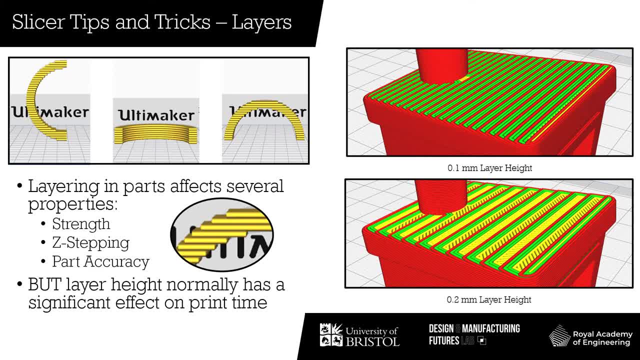 Generally, you'll see an increase in part strength for increased layer height, most notably in cases of tensor loads applied perpendicular to the layers, ie the z-axis of the print. Lots of information is available on this online and in research, As already discussed. 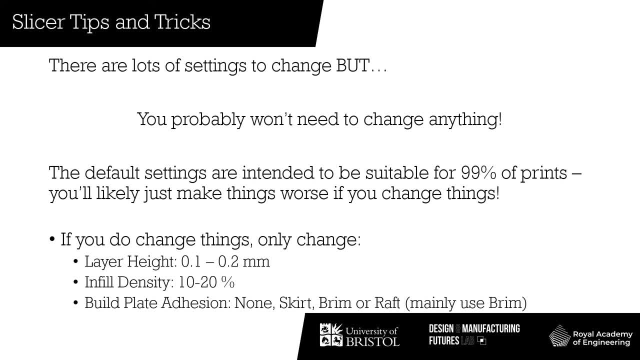 the parameters and model you input into a slicer will directly influence the resulting print output and follows the adage garbage in equals garbage out. As such, it is vitally important you consider the model generation and parameter decision process carefully. Thankfully, much of the 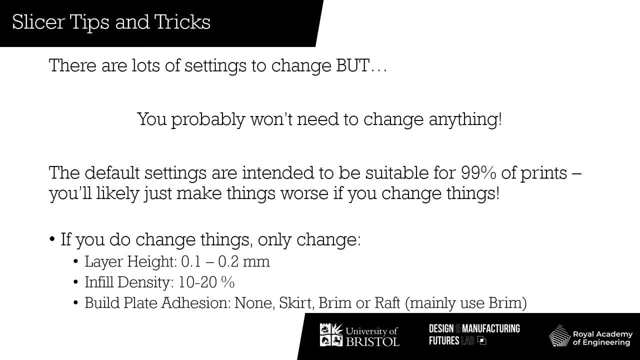 hard work is already done for you and therefore I highly recommend you don't change anything from the default printer profiles provided in 99% of cases. It is likely you'll just make things worse or forget the change in back for your next print. 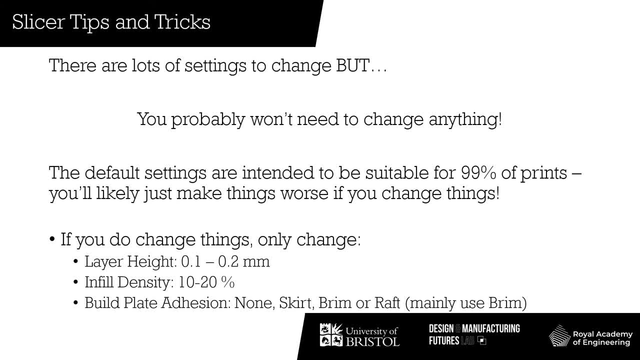 If you do change settings, I would suggest you limit yourself to layer height, infill density and build plate adhesion method. If you have a particularly strong desire to change anything else, I'd recommend you have a robust process of confirming why this is particularly important and discuss this with the 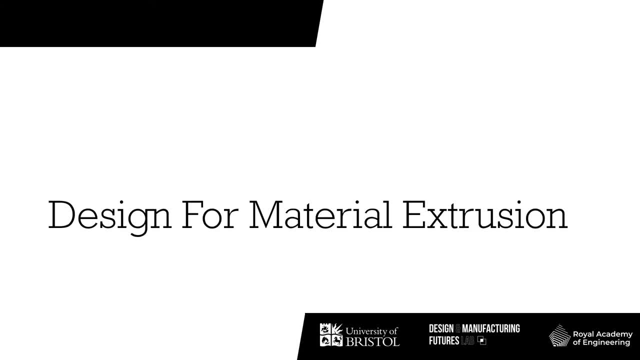 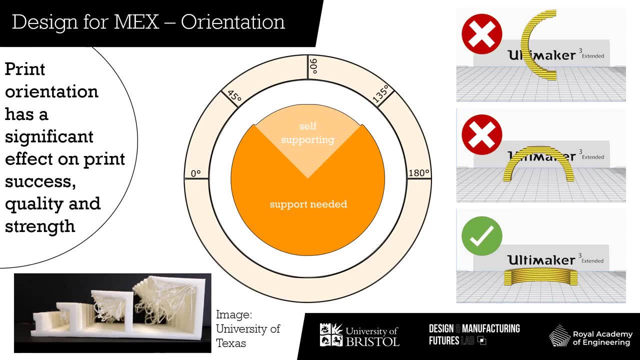 technicians or machine owner. before trying anything Along with the slicer tips and tricks regarding print parameters, you need to carefully consider what you design for MEX printing. Due to the nature of layered manufacturing methods, it is generally important that layers are supported from beneath to avoid partial or 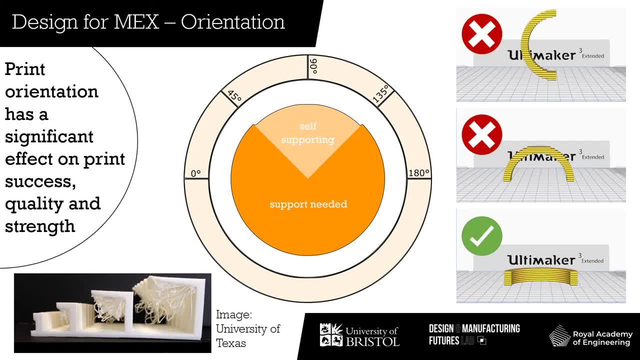 total collapse. As such, one of, if not the most important considerations when designing a part and slicing is model orientation relative to the build direction. By considering model orientation whilst designing products, you are able to reduce the amount of support required when printing. 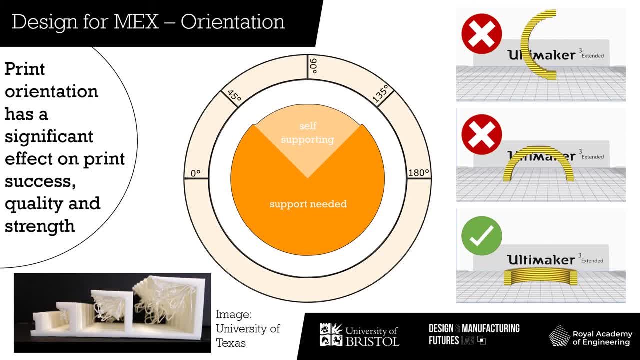 that often doesn't perform that well, slows the print down and requires post-processing while simultaneously improving part accuracy and print success rate. It is, however, recognised to that it may not be possible to have no overhangs or unsupported surfaces, and that's why we have 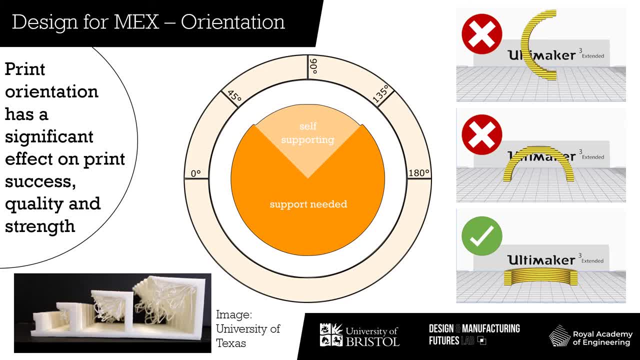 the 45 degree rule of thumb. If possible, all surfaces should be supported at a minimum by a chamfer within 45 degrees of the vertical axis. This can be easily placed in most CAD applications as a feature, with an angle and distance parameter Where possible. 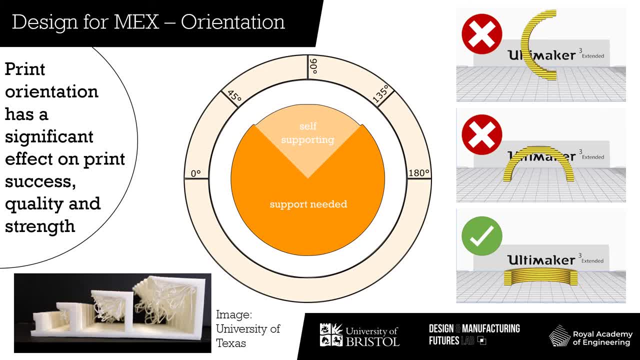 you should ensure the chamfer angle is as close to vertical as possible, as this will improve the part accuracy and chance of print success. Print orientation also has a significant effect on part strength in different directions If you know the loading direction of your part. 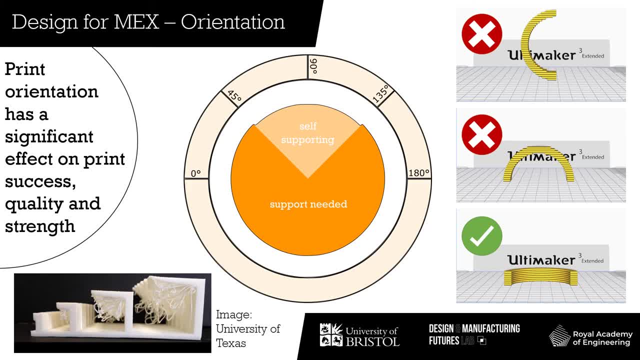 which you should. you will want to orientate your part such that layers run parallel to the load direction. This means that you should avoid loading your part in tension along the z print axis, as you will otherwise find that you are pulling the layers in your part apart. 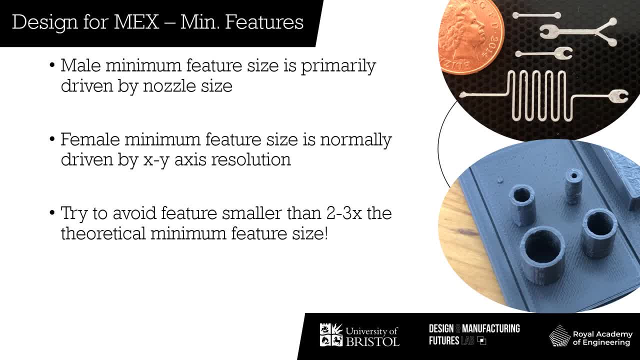 causing premature failure. Another important consideration is the minimum feature size used in your model. To decide on this value, you need to consider the printer you are using and a resolution on the xy-axis and a resolution on the xy-axis For minimum geometry of male features, ie features that stick out of your part. 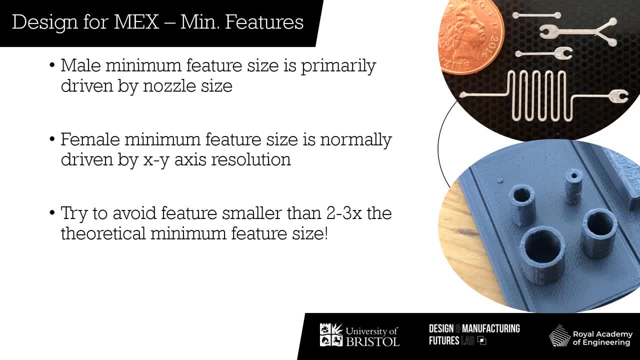 you will likely be limited by your nozzle size above any other factor, with the nozzle diameter likely to be a magnitude or more greater than the resolution of the xy-axis. Building male features smaller than the nozzle diameter is a near impossible task, as you are generally unable. 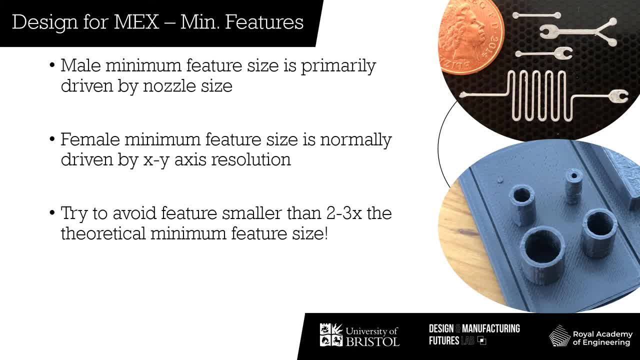 to control the material flow rates carefully enough to allow for smaller extrusions. When working out minimum geometry for female features, ie features that are assessed into the part, you will need to consider the xy resolution over any other factor, though the nozzle diameter can also have an effect depending on how the slicing software develops the print. 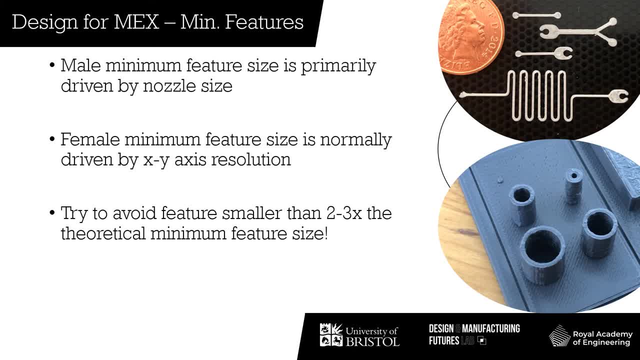 paths and places the nozzle. Generally, it is easier to get finer resolutions for female features than male features. Minimum feature size in the z-axis is normally limited by the layer height more than any other factor, as the features can only be printed in multiples of the. 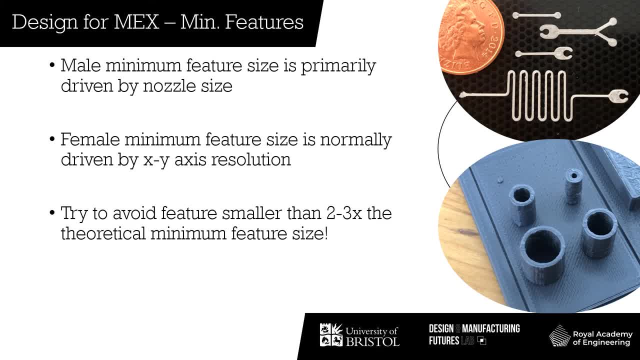 layer height, As such features can sometimes be significantly different or, in some cases, completely missing. The location of the features in the z-axis are also more important for features in the x- or y-axis for the same reason, and should be designed such that they start at a. 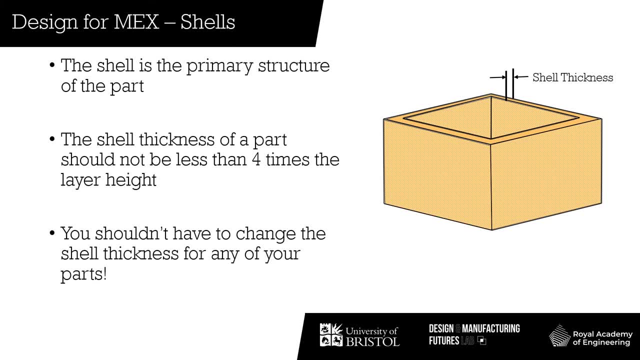 layer intersection. The shell of an MEX fabricated part is its primary structure and is therefore very important in defining the part's accuracy, strength and aesthetic. Generally, the default shell thickness is perfectly fine for any application and should therefore not be changed. 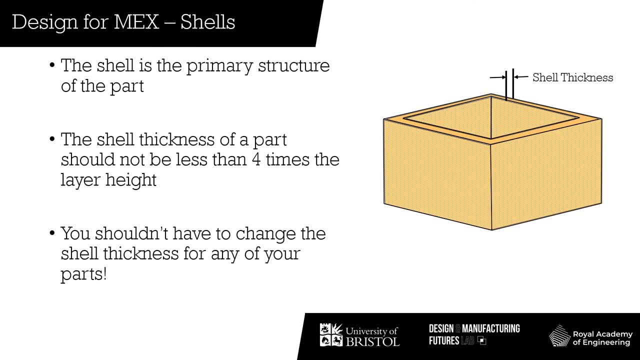 However, it should be considered when designing a part such that you don't require surfaces that are 4 times the expected layer height, as this will cause several issues. In most instances, this means you should aim to not have walls narrower than 1mm in your design. 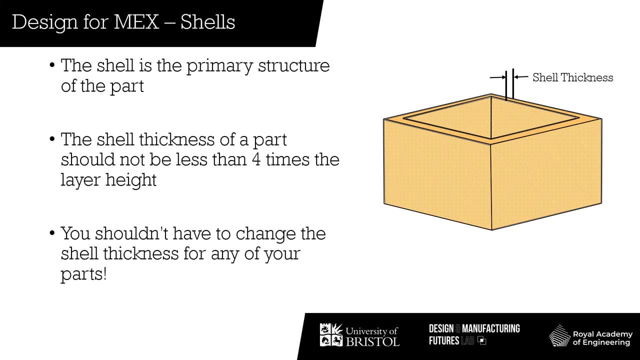 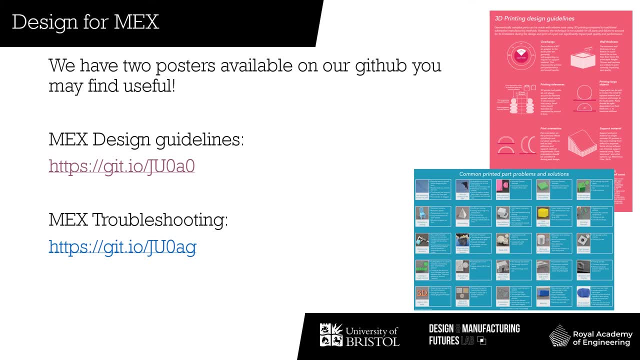 This rule applies for all external geometry, including side walls, top layers and bottom layers. There are lots more design for manufacturers associated with using MEX printing that should be considered, and two of our team have produced a summary of the key ones in a. 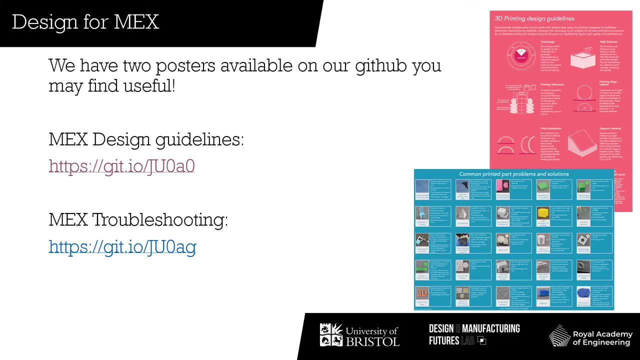 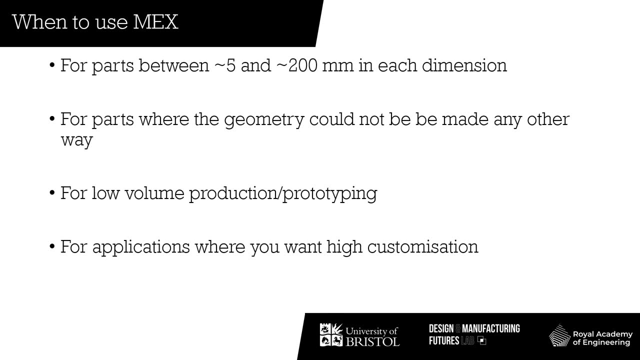 poster now available on our github. As well as this, they have also created a general troubleshooting guide for issues commonly encountered when using a technology that are available from the links you can see. Please feel free to use these as appropriate. Although MEX offers many advantages, it is important to consider when it is suitable. 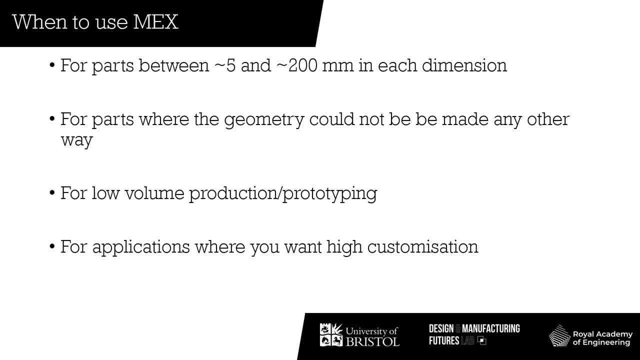 to use the technology as it is with all additive technologies. For normal desktop machines, applications should be intended to be between 5 and 200mm in any direction. Any smaller and you won't get consistent results, and any larger and you'll likely suffer lots of. 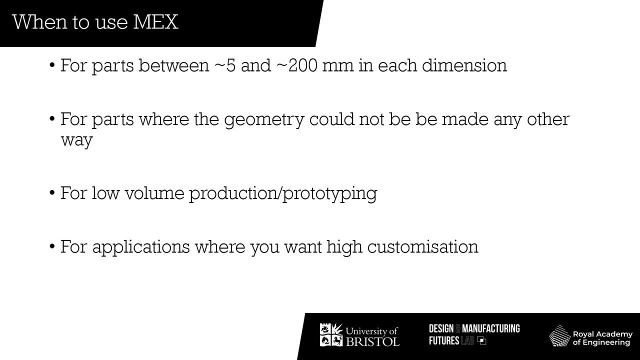 print failures and be waiting a long time for parts. Of course, the ability to use the MEX technology will not be a problem if you are using it for a limited time. The ability for the printer to print almost any geometry is particularly useful. 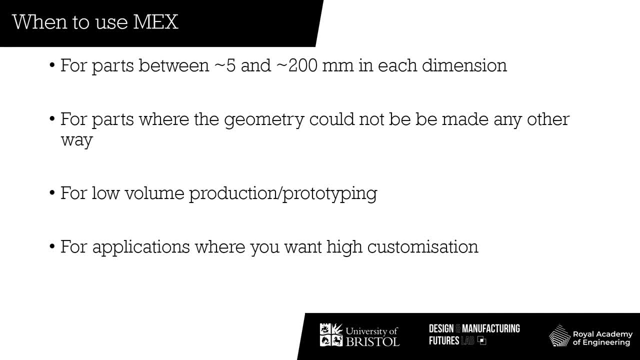 and, as such, the technology should be used when you are unable to manufacture geometry in any other way. In applications requiring low volume MEX printing, it is also likely to be advantageous, as the long print times are offset by the time required to produce tooling or generate complex 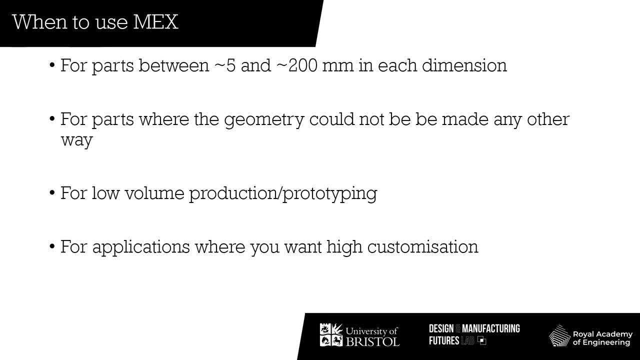 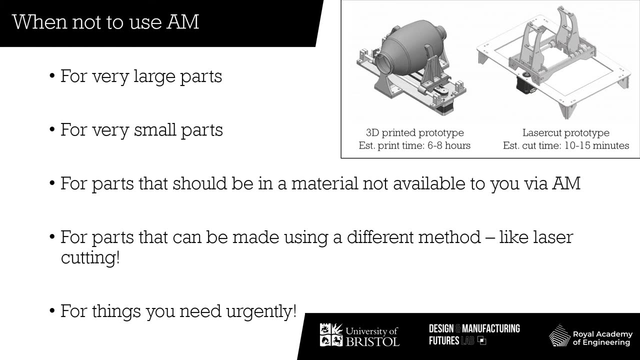 machine parts. And finally, MEX printers offer the ability to provide highly customisable designs, as no tooling is required. As such, it is a very useful technology when designing parts or prototypes with a lot of cost. In contrast, there are many instances in which using MEX printing- or any form of 3D printing for that matter- is unlikely to be helpful. 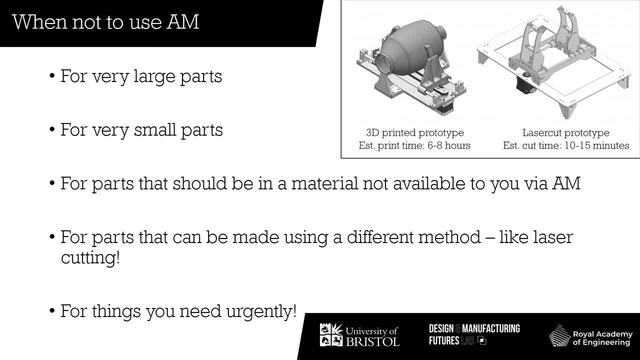 As previously discussed, the technology isn't very useful for very large or very small parts without significant modification and should therefore be avoided. when dealing with these geometries, You'll also find that most of the desktop printers you have access to will likely be suitable for plastic prints only. 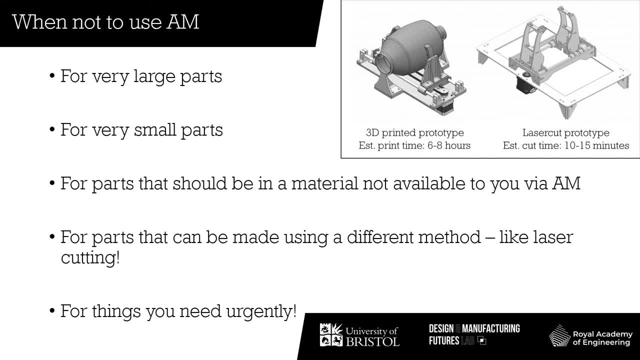 and so the technology should be avoided when one of the available plastics is not suitable for the application. ie gears that should be made out of metal should not be printed in plastic. you'll only find lots of issues if you do this. Other manufacturing methods should also be considered, as they are often quicker, cheaper and easier. 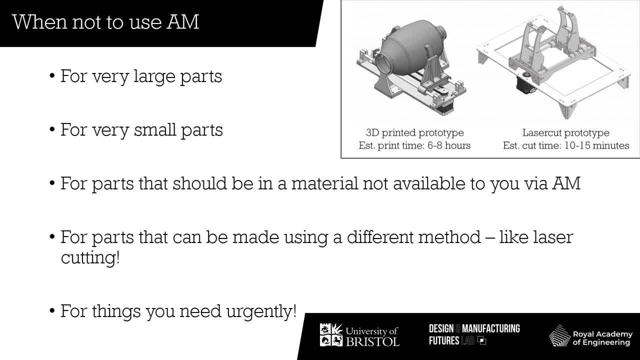 The laser cut example of a rapidly developed ventilator from our group in response to the COVID-19 pandemic can be manufactured in 10-15 minutes, compared to 6-8 hours for the equivalent 3D printed version, Even if you don't have access to things like laser cutters. 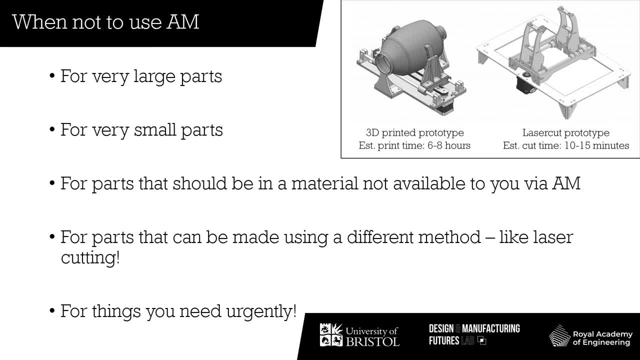 consider whether cutting up some cardboard using lego or junk modelling or even virtual methods would be appropriate, as, as the last point notes, MEX isn't great if you need things urgently. Now we've covered a lot of information very quickly in this video. 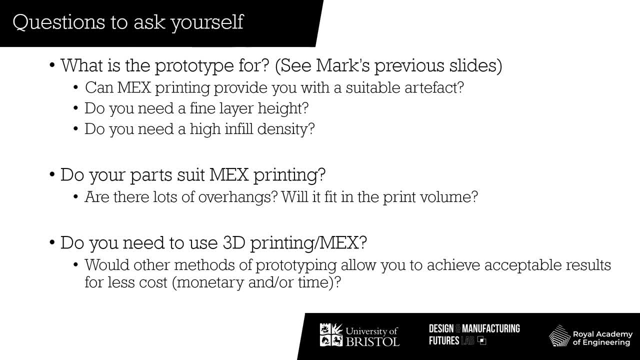 which I appreciate you aren't likely to remember all of when prototyping and considering MEX printing As such, we've derived three questions you should ask yourself. that should hopefully make this a little easier. Firstly, what is your prototype for? Is your prototype intended to be a replica? 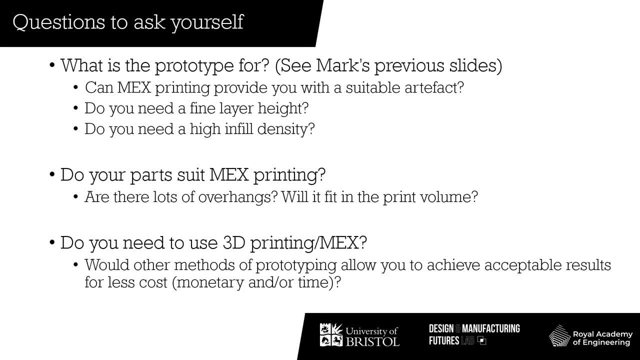 of the final product and function as such, or is it just to look at? Do you care if you have an error of a few millimetre in each direction? Look at Mark's prototyping video if you're unsure on this. Secondly, does your geometry suit 3D printing? Have a look back at this video, as well as the. 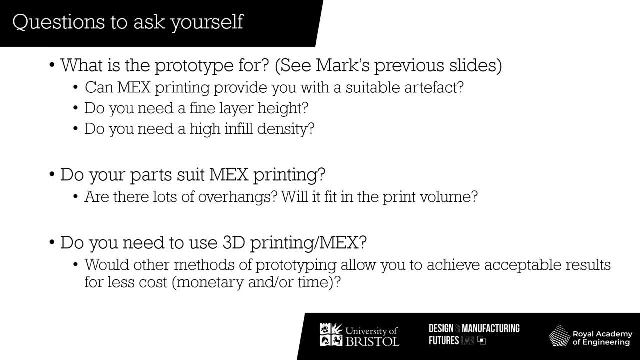 3D printing design guideline poster. if you're unsure, If the answer is no, why not? Can you fix this If you can do? If you can't, you'll need to consider the implications, and I would suggest. your speedster is responsible for organising and running the printer you plan on using.